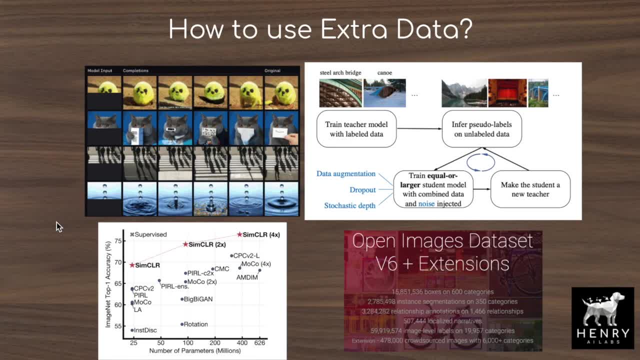 not. This paper is addressing the question of how do we use extra data, whether it's labeled or not, particularly for the downstream tasks of object detection, where we assign a bounding box over an object of interest in an overall image, or semantic segmentation, where we classify every single pixel in the image. 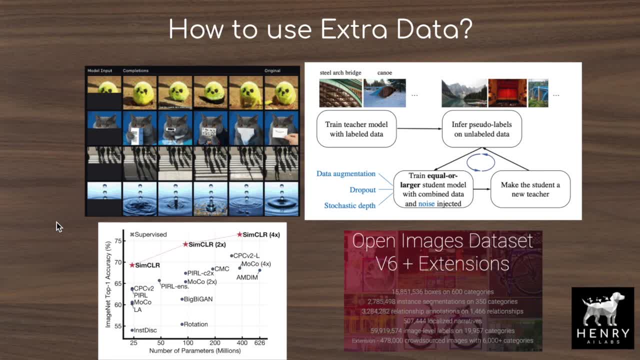 So we'll start off with the clear supervised transfer learning. That would be where we take a model and train it on a large labeled dataset like ImageNet and then we repurpose those features as the backbone for an object classification head to be trained on top of those features. 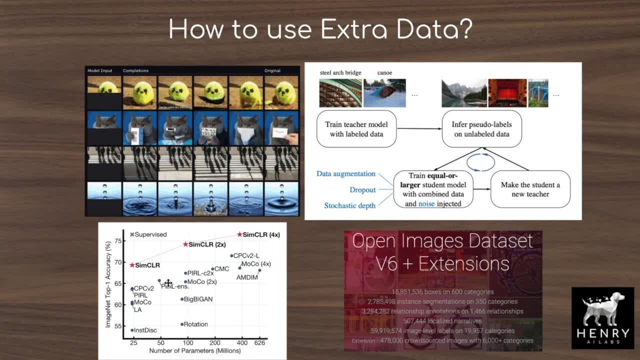 Another technique is self-supervised learning. So here are two different ways of doing this. You could have a technique like SIMD, which is a self-supervised learning technique, or a self-supervised learning algorithm called SimCLR. SimCLR is a contrastive self-supervised 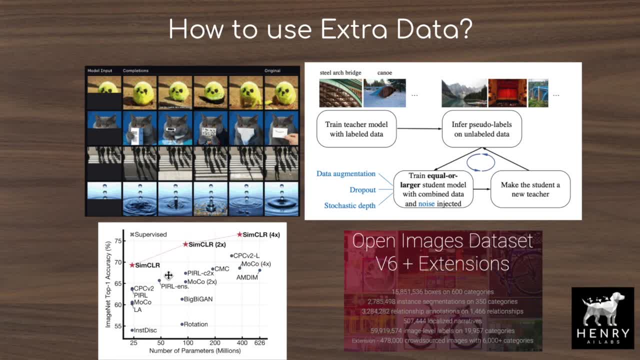 learning algorithm and it learns representations by making the representations of an image similar to a data augmentation view of that same image and dissimilar to all the other images in the training set or some batch, like the queue used in momentum contrast. So these contrasted. 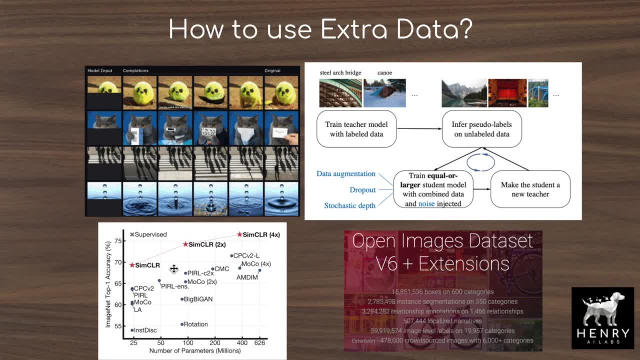 self-supervised learning algorithms have been pretty successful, with SimCLR version 2 coming out very recently as well. Another strategy for using self-supervised learning to leverage extra unlabeled data would be the strategy in ImageGPT, where you train a generative model on this massive 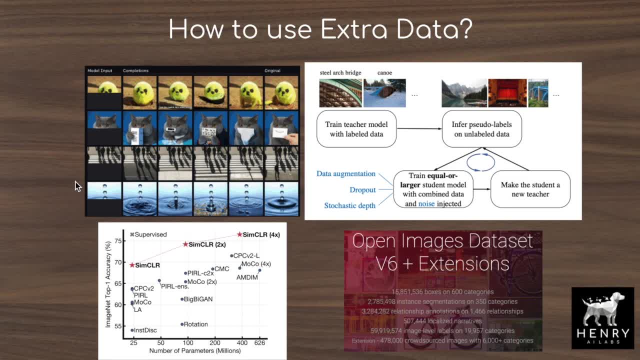 unlabeled dataset and then repurpose those representations to fine-tune for, say, ImageNet classification or, in this case, COCO object detection or Pascal semantic segmentation. So the third technique that is going to be shown to be very effective in this paper, 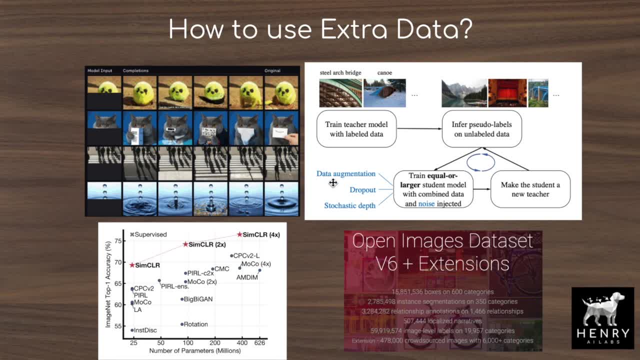 is self-training. Self-training was made really popular with the self-training with noisy student paper that achieves the ImageNet classification state-of-the-art. So it's this technique that I'm going to describe in more detail in the next slide that uses the unlabeled data with the smaller. 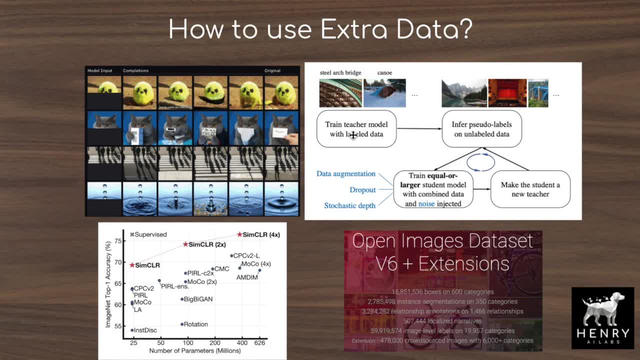 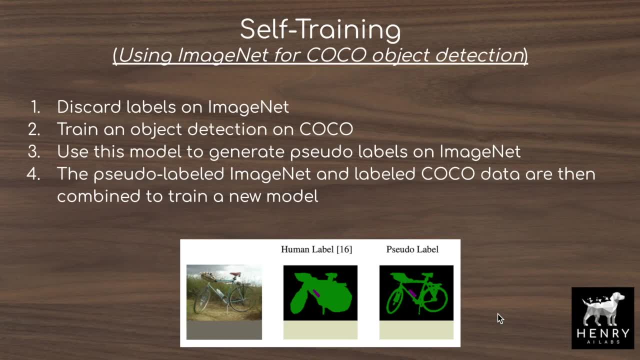 set of labeled data simultaneously throughout training to improve upon the signal in the labeled data by leveraging the unlabeled extra data. This is the idea of self-training in the example of using the ImageNet dataset to help with training a object detection model on the COCO labeled dataset. So COCO is this dataset of images that have bounding boxes over objects like 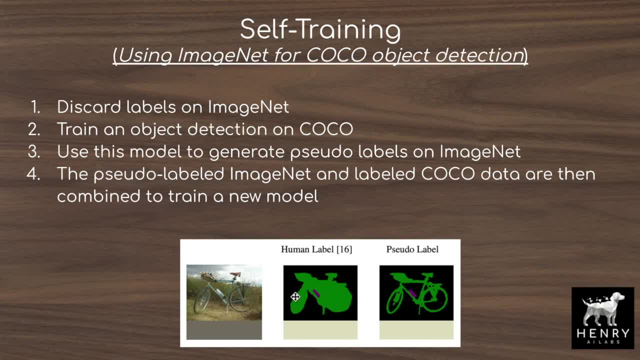 this bike. This example is semantic segmentation, where we're labeling every pixel in the image as the semantic class, like bike or background. so the first step of self-training is to take the larger data set and if it's already labeled, like in the case of imagenet, we throw away. 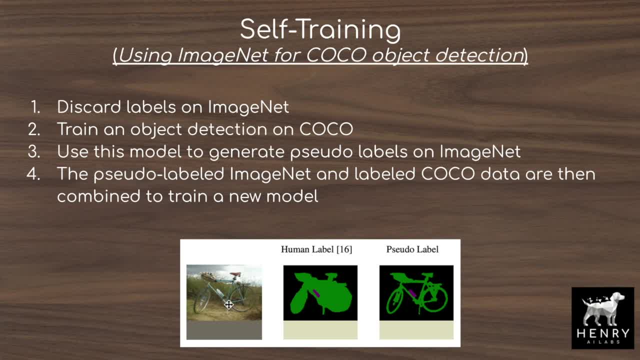 these labels, because we're not going to be taking this bike image and just mapping it to bike. we're going to be trying to design the bounding box across the bike, so then we're going to train the object detection model on the labeled coco dataset, so then we take that model. that was. 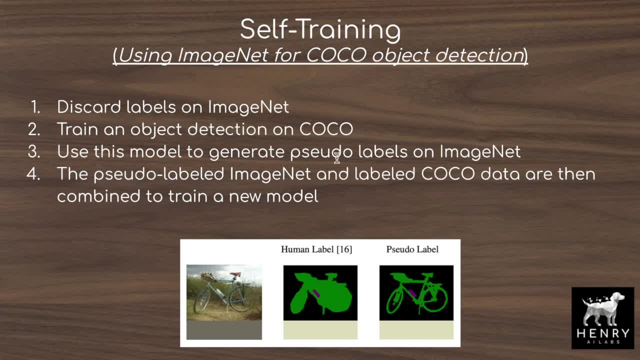 trained on the coco dataset and we use it to generate pseudo labels on imagenet. so this means taking each of the images in imagenet and then putting them through a forward pass of coco and having them come out with some pseudo-labeled bounding box that this model has predicted on. 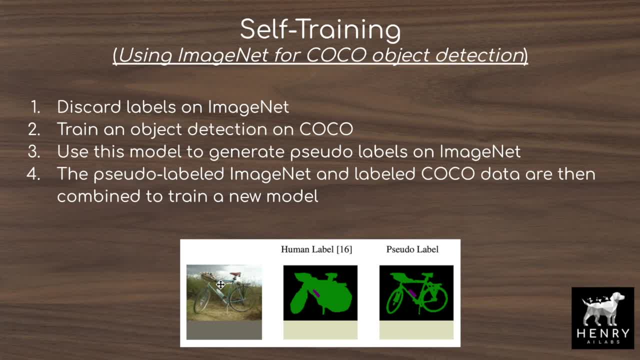 the image. so in the case of semantic segmentation, you see the example of the model train and the limited labeled semantic segmentation data set and then it takes the imagenet image and produces this new pseudo label for it. so then you're going to aggregate the pseudo labels at this iteration step. 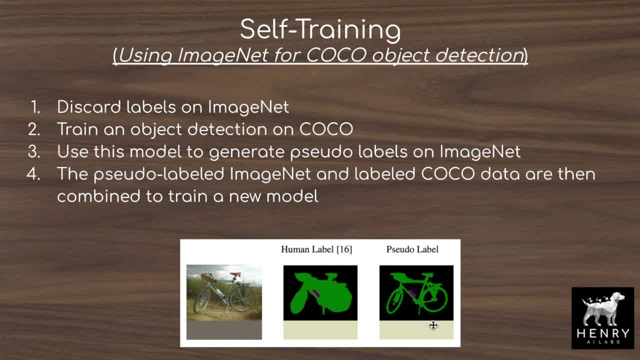 and the labeled data set and use that to train a new model that's been randomly initialized. so it's a bit more computationally expensive to do self-training with these iterations of training the model, but it performs better than pre-training- either supervised pre-training or self-supervised. 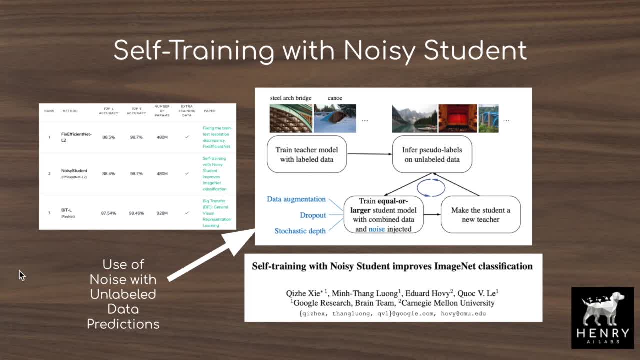 pre-training. another factor of the self-training pipeline, especially what's used in noisy student, which achieves the imagenet state-of-the-art at 88.4 percent top one accuracy is to inject noise when the model is pseudo-labeling the unlabeled data set. so this noise can be in the form of doing. 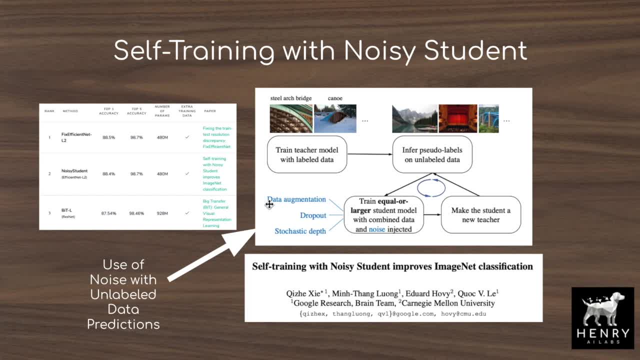 data augmentations like rotations, translations or color alterations to the unlabeled data image, or applying dropout in the model or stochastic depth, which is where you drop out an entire path of the network. so you integrate this noise with the prediction on the unlabeled data to add some more robustness and add more signal with respect to applying these pseudo labels on. 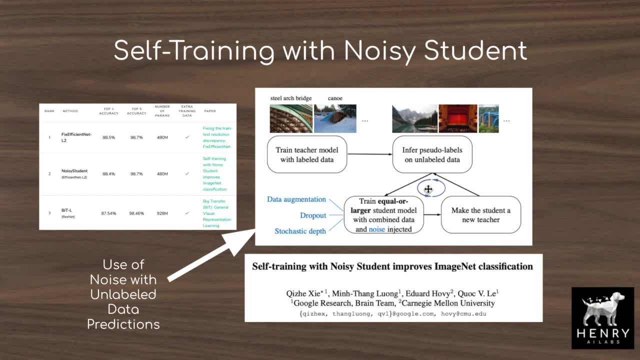 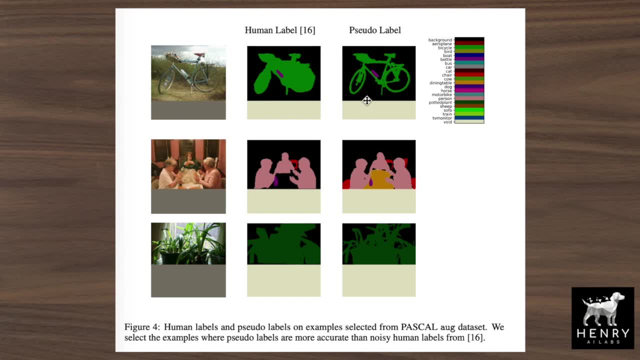 the unlabeled data and then stacking the pseudo-labeled data sets with the label data to train the next iteration of a model. these are some examples where the pseudo labels that come from the model trained on the limited data set is able to perform a more precise labeling of. 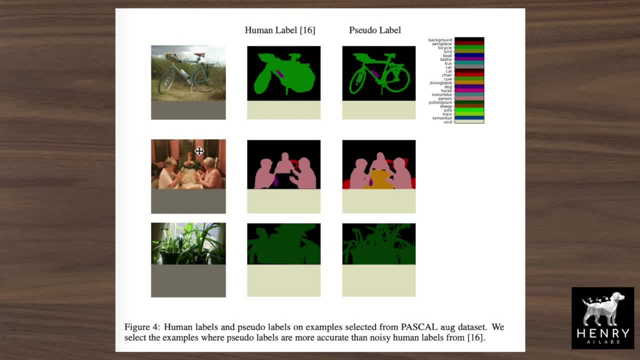 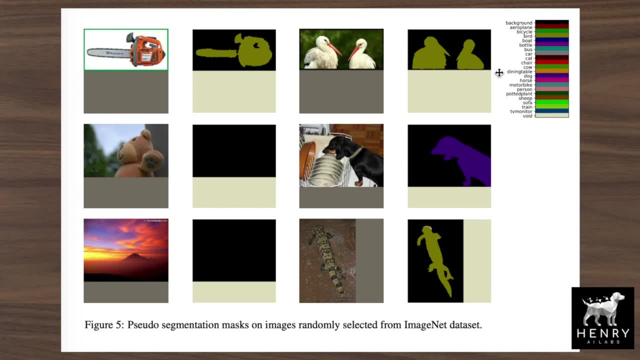 the image than the human labelers. in this bike image, eating dinner image and then this plant image, you see more precise labeling with the pseudo label from the previously trained model, and these are cases where the pseudo labeling fails. you see, in the bear image there's no. 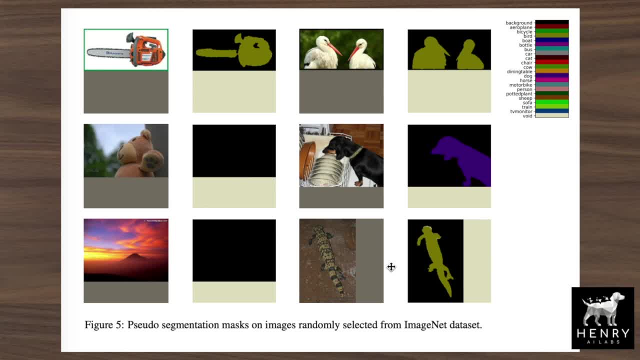 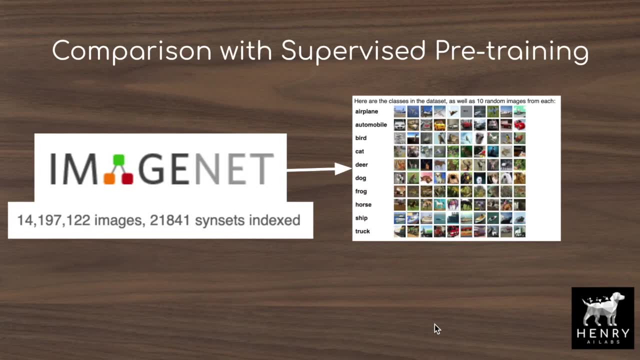 highlight at all. it's just all black, as is the landscape image, and these other landscapes aren't quite as precise as the ones in this example. so we're comparing the self-training paradigm with supervised pre-training and self-supervised pre-training. so supervised pre-training describes 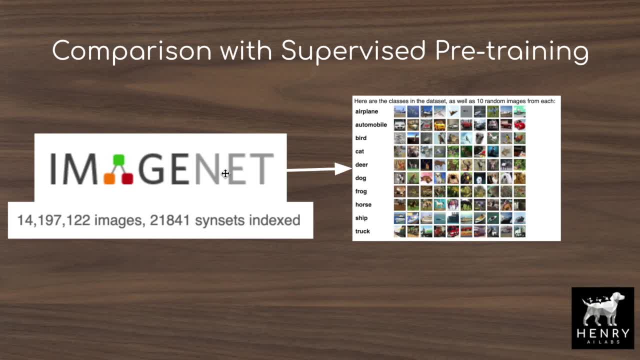 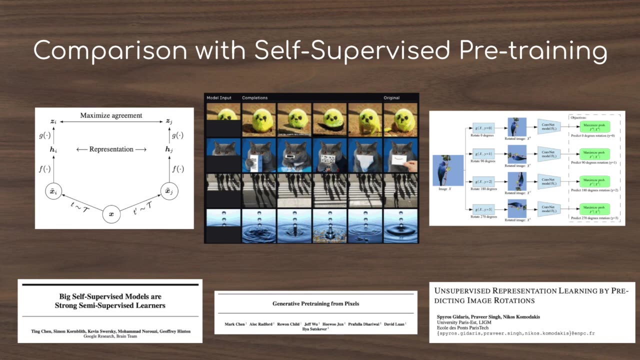 pre-training, the model on the imagenet labeled data set, where we have the cross entropy loss over class predictions, and then we would fine-tune these features on a downstream task like cfar10 classification or coco object detection, pascal semantic segmentation. so the next comparison is with self-supervised pre-training. so this is another really. 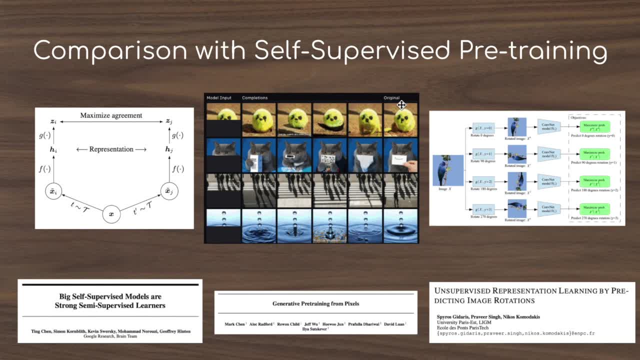 popular technique to make use of unlabeled extra data. so the first class of techniques is contrastive self-supervised learning. so these are techniques like momentum contrast, contrast of general unit sum data, and the second class of techniques of instance, nanometric decoding and sim clr. so simclr takes an image and then augments it to perform two views of that same image and 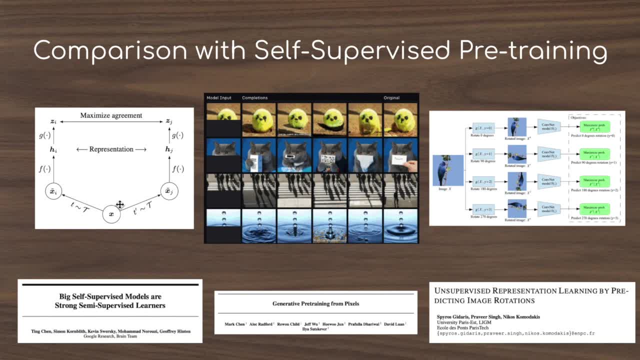 then the representation between these two augmented images are optimized to maximize their agreement. so there are all these other techniques that try to push representations of the same image and augmented views of it towards each other and then dissimilar from other images in the mini batch data set, or q, as in the momentum contrast algorithm. so the next technique would be: 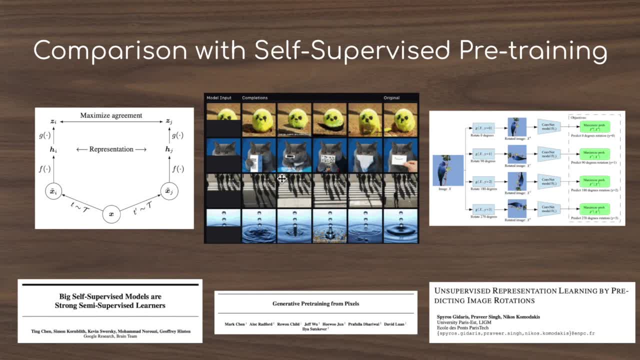 learned by the generative model for a downstream task like COCO object detection. So really famously, ImageGPT just released their paper with 6.8 billion parameters where they train this autoregressive pixel prediction model that can perform pretty well on ImageNet classification. 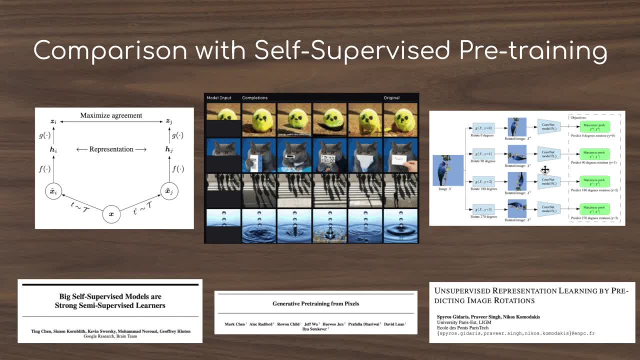 Another way of doing self-supervised pre-training would be to construct an auxiliary or some kind of artificial supervised learning task, like rotating this image 0,, 90,, 180, or 270 degrees and then predicting the rotation angle on the made-up task. 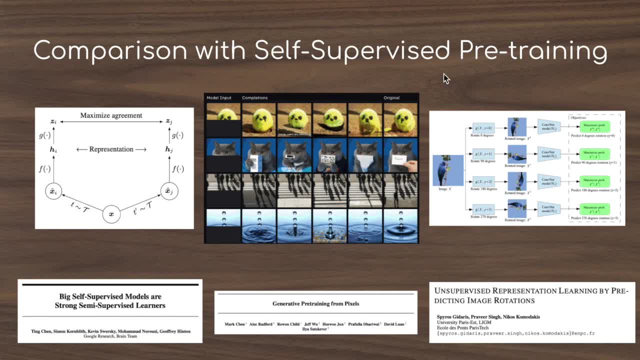 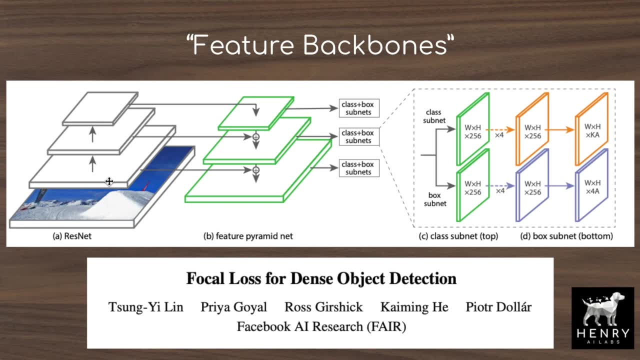 and then using these representations to fine-tune for COCO object detection, The authors experiment with the retina net architecture. So the way that this works with, say, supervised pre-training or self-supervised pre-training, is you will take this feature backbone that takes in the raw image. 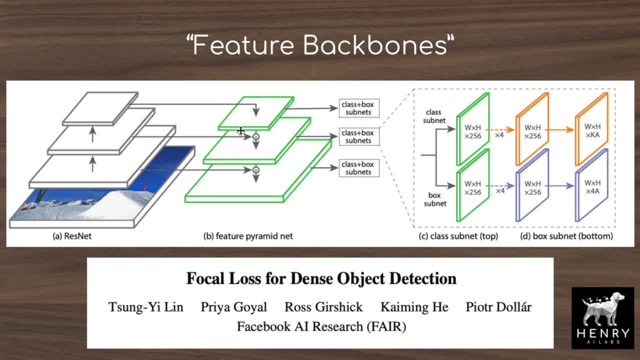 then extracts these levels of features and then you'll pipeline this into a feature pyramid network. These feature pyramid networks are used in object detection and semantic segmentation to get the multiple resolution scales of the feature maps. Because convolutional networks, they downsample the height and width of these feature maps as they go through the network. 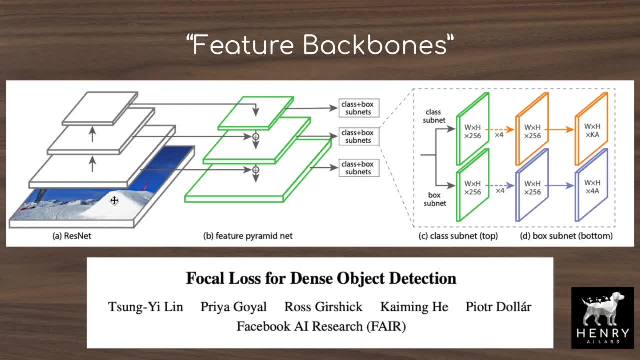 So this might be the 256 by 256 ImageNet image and this might be 128 by 128, 64 by 64, and then 32 by 32.. So you use this kind of feature pyramid way of going down and pooling the feature maps. 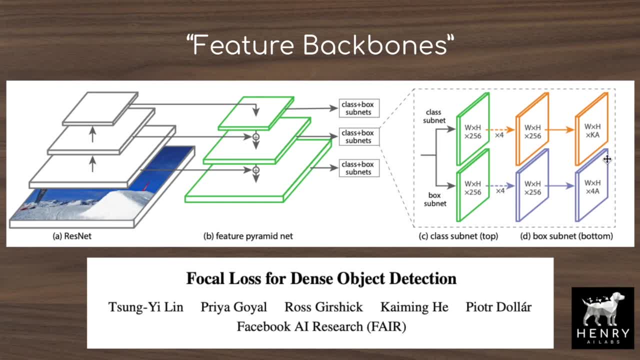 in the intermediate feature backbone to pipeline this into the classification head at the top, that does the bounding box regression loss on the coordinates of the bounding box as well as the actual class, like bike, elephant or whatever it's trying to classify. So there's a lot of different architectures for object detection. 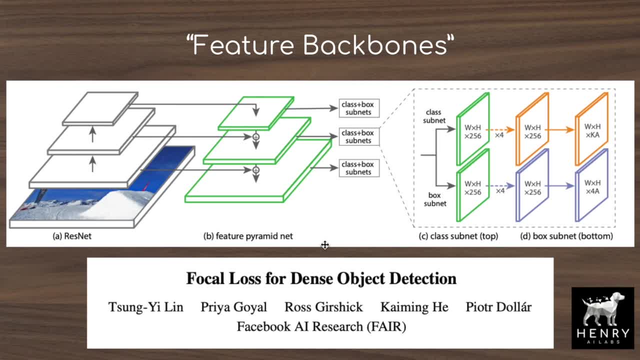 Most recently, the debtor model from Facebook uses a set kind of loss function. that's a lot different from this kind of paradigm with the transformer architecture, But this is the model architecture that's being explored in this paper, also similar to the efficient debt model. 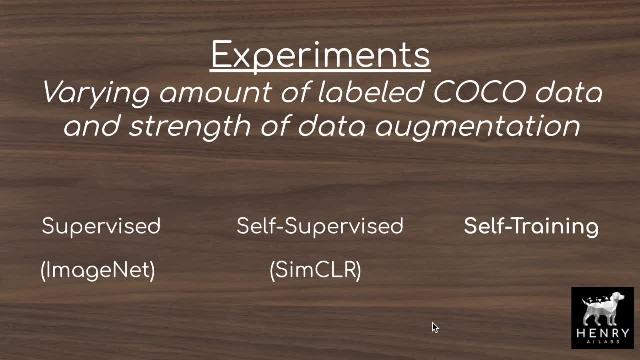 So the first set of experiments we'll look at are varying the amount of labeled COCO data. So this is the amount of labeled data for the downstream fine-tuning task and then the strength of the data augmentation used. So they're experimenting with data augmentation. 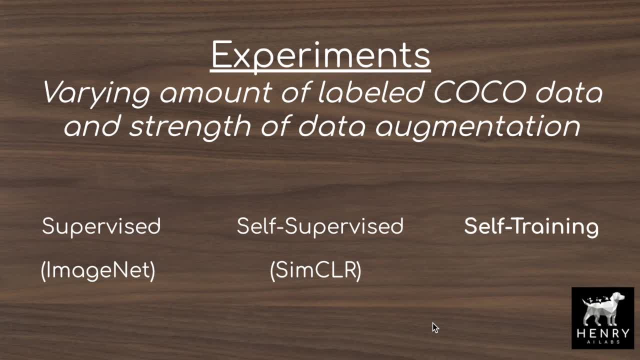 like simple flipping or things like auto augment or rand augment, that have more sophisticated ways of scheduling the magnitude of data augmentations, like whether you're going to rotate it 50 degrees or, say, five degrees, and scheduling how you're going to do that throughout the training. 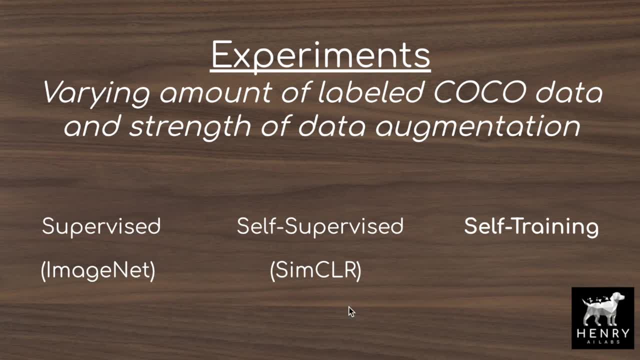 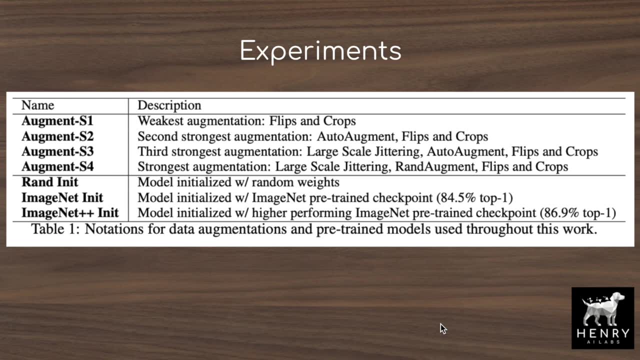 So they're comparing supervised pre-training with ImageNet, self-supervised learning, particularly with the SIM-CLR contrastive learning algorithm, and then the self-training algorithm described previously. The experiments are controlling for the amount of augmentation or regularizing noise that's used in the fine-tuning. 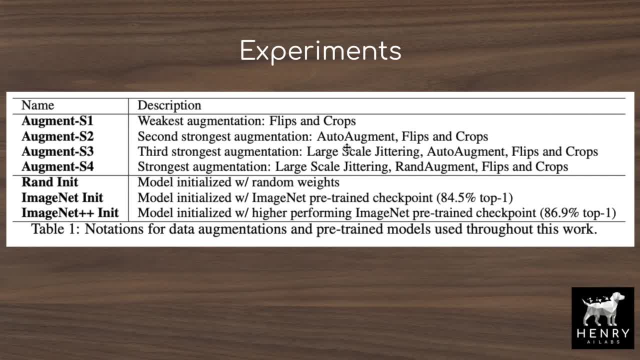 whether it's the simple flip, flipping and cropping augmentation using auto augment, large-scale jittering plus auto augment or large-scale color jittering plus the rand augment. automated scheduling algorithm, differently from auto augment. So then, with respect to the supervised pre-training initializations, 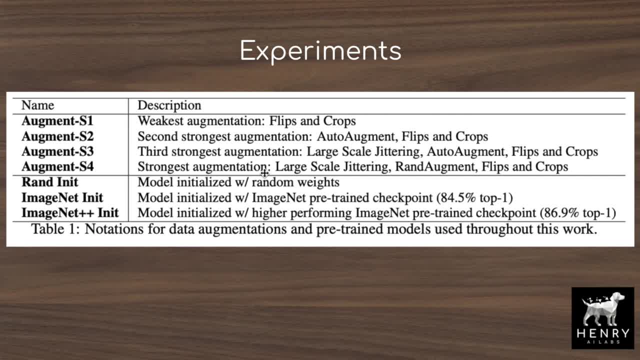 they experiment with a model initialized with random weights and rand in it. ImageNet in it is a model that's been pre-trained with the auto augment and the ImageNet labels and achieves 84.5% top-one accuracy on ImageNet and ImageNet++ in it. 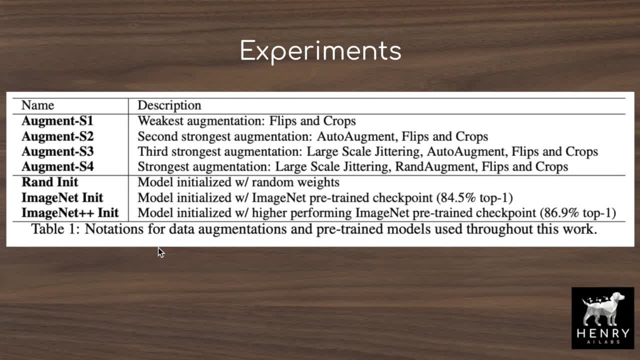 is the model that's been pre-trained with the auto augment and the ImageNet labels and achieves 84.5% top-one accuracy on ImageNet, which is the model from self-training with Noisy Student that uses an additional 300 million images from the JFT data set. 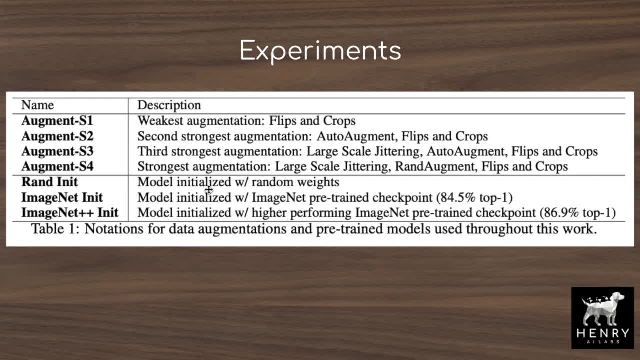 So in ImageNet in it and ImageNet++ in it, they're controlling for the model capacity. These both use the EfficientNet B7 or L2, not sure exactly the variant, but they're using the same model capacity and they're just controlling for how well the different models are performing. 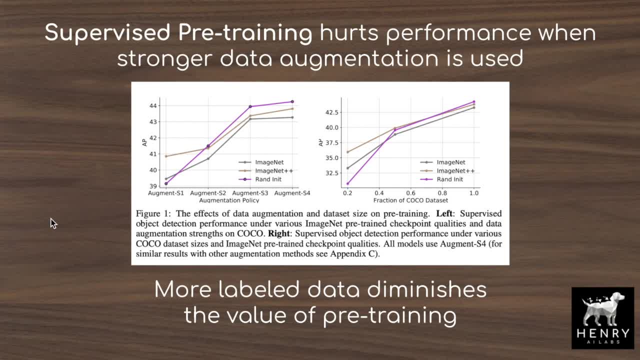 at the pre-training supervised learning task. The first set of experiments shows that supervised pre-training hurts performance when stronger data augmentation is used. So the purple chart is the random initialization and then the orange is the ImageNet with the self-training, with Noisy Student. 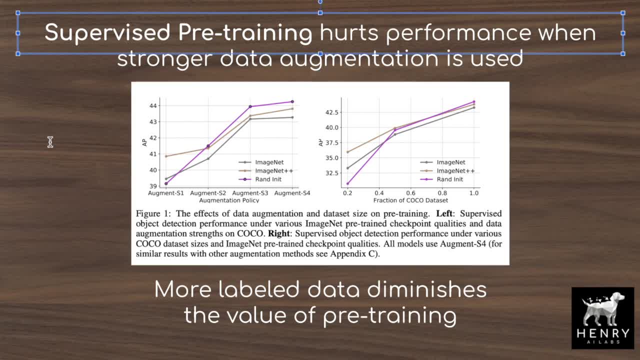 weights at 87% accuracy and the gray one is with 85% accuracy. You see, as more augmentation is being used, only the random initialization model is really improving with the average precision metric compared to the supervised pre-training models. So at the small scale of data augmentation where you're just flipping, 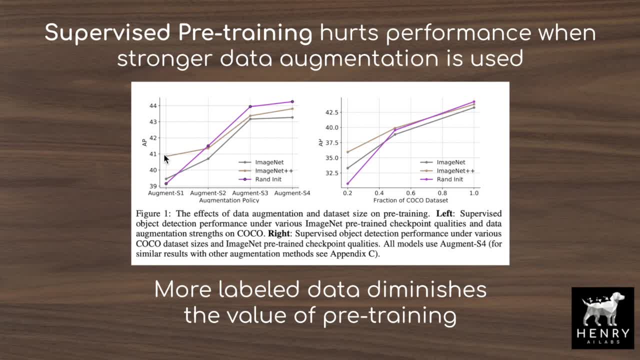 the images. the EfficientNet with the 87% accuracy performs better than random initialization. As you scale up, the random initialization performs better. And then this shows that once you increase more data, the pre-training with the supervised learning becomes completely useless in the case of only 20% of the labeled COCO data set for the downstream. 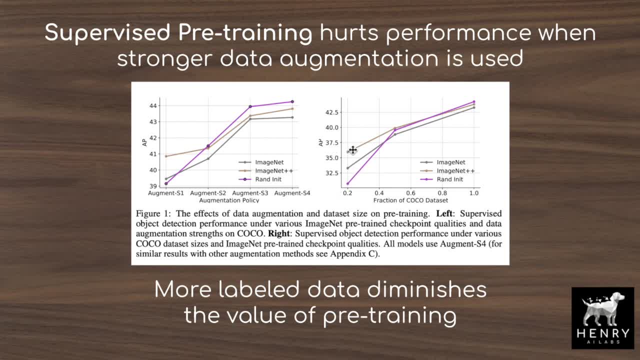 fine tuning task. you get better performance with the 87% ImageNet accuracy feature, extracting backbone. But once you start adding more data, all these lines blur and become the same, with the random initialization performing about better. The next table shows that self-training helps in these cases where strong. 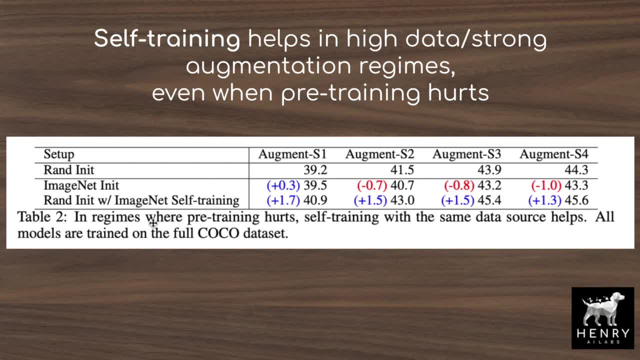 data augmentation is causing the ImageNet pre-trained model with supervised learning to decrease performance, even surpassing the random initialization. So this is the performance of the randomly initialized model as it starts to increase with more data augmentation and the supervised learning model starts to decrease or it still improves. 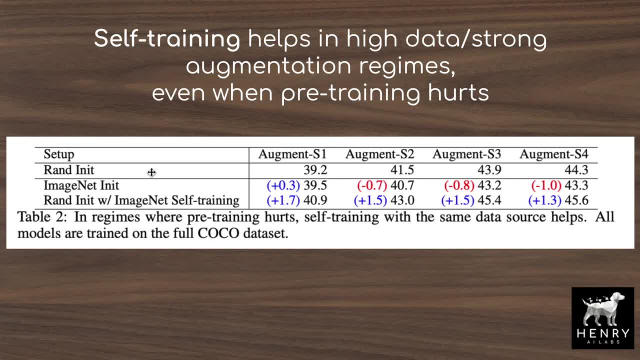 but not at the same pace of the random initialized model. But when you also do the ImageNet data set for self-training. so you're fine tuning the randomly initialized model on the small labeled COCO object detection data set and then you're treating the 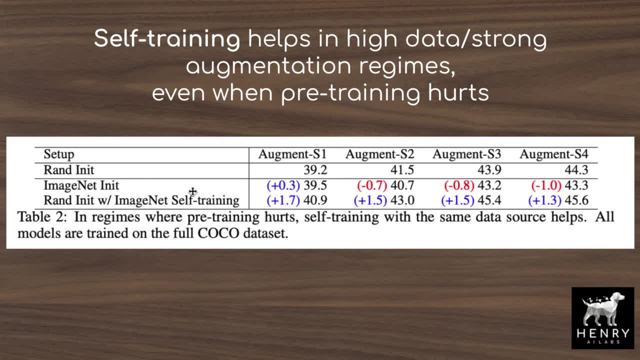 image net data set like it's a object detection data set, and you're labeling it artificially with the model trained on the subset of the COCO labels. And this is continuing to improve, more so than the random initialization, as you increase the strength of the data augmentation. 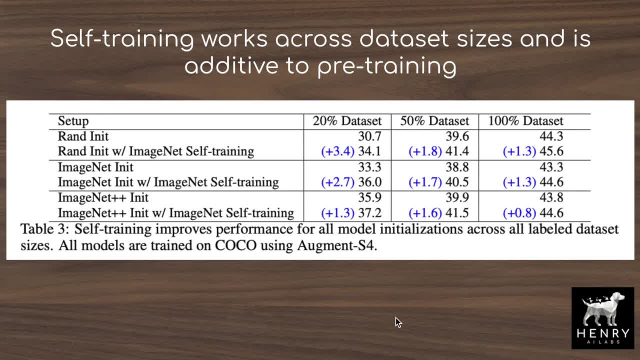 This table shows that, even when we're increasing the amount of labeled data for the downstream fine tuning task, self-training continues to improve the performance even with 100% of the labeled data set, whereas the random initialization is starting to surpass the ImageNet supervised learning. 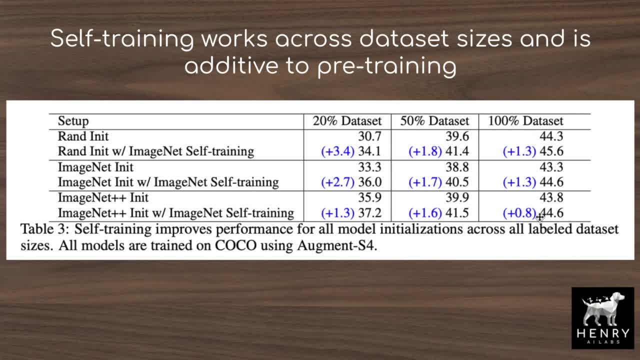 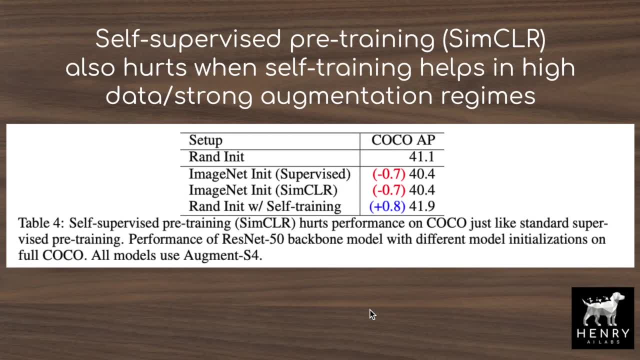 pre-trained model to start out with. So we're seeing that self-training is additive to this random initialization and continues to improve, even when you add more labels for the downstream task. Self-supervised pre-training with the SIMCLR contrastive representation learning algorithm also hurts in the case of the higher augment S4 data augmentation. 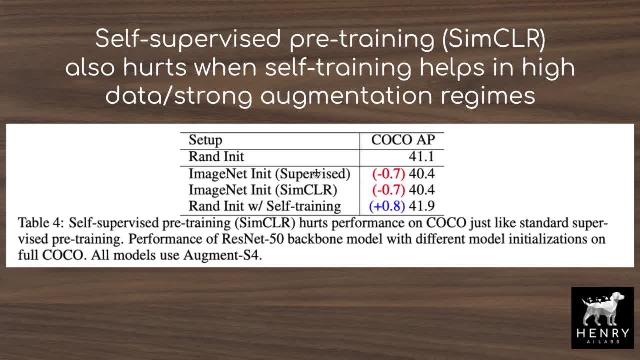 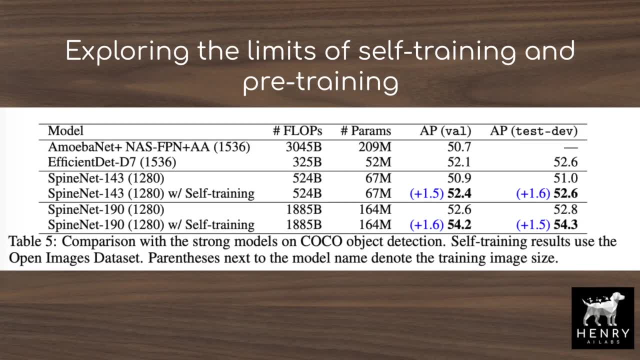 in a similar way as the supervised learning initialized weights. So we're seeing that only self-training is continuing to improve on the performance at the higher levels of data augmentation. The authors further investigate the gains that can be achieved with self-training and pre-training by using 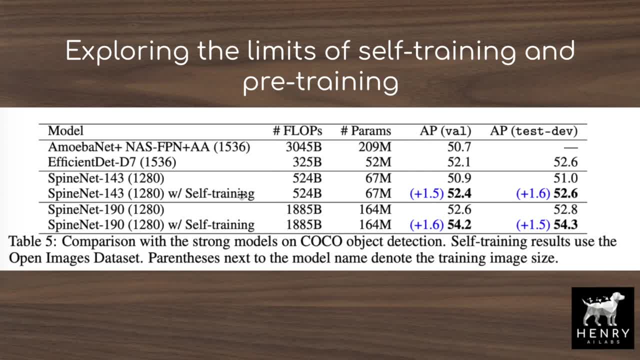 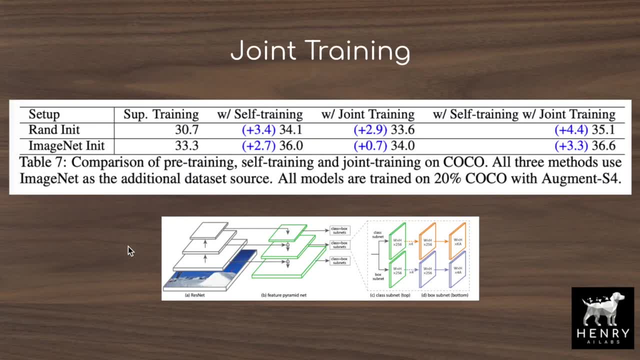 the open images data set to do the self-training or have this unlabeled counterpart with the labeled data for COCO object detection and the Pascal semantic segmentation data set. The authors further explore stacking these techniques together with joint training. So joint training would describe also doing the image classification and 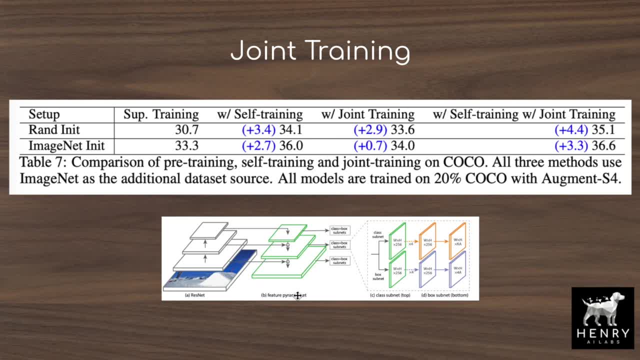 simultaneously passing the gradients through the object detection loss. So we see the baseline performance with just the supervised training, where we just train with the limited COCO data set and we're doing object detection. Then with self-training where we're doing the COCO classification and we're also using ImageNet as additional data to 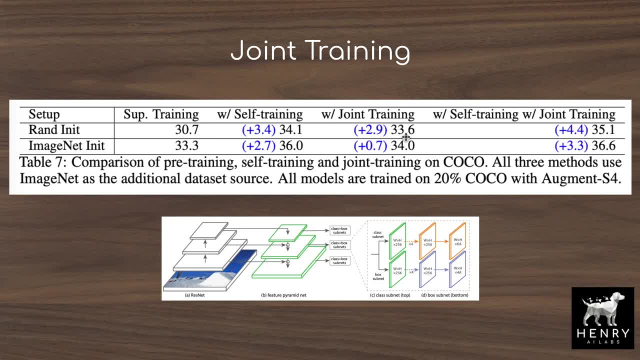 supplement our pseudo labels for the self-training pipeline. Joint training would describe simultaneously doing ImageNet classification with this feature backbone and doing the object detection. Now we can also do self-training and the supervised training and the pre-training supervised training, so we could train this feature backbone on ImageNet classification. 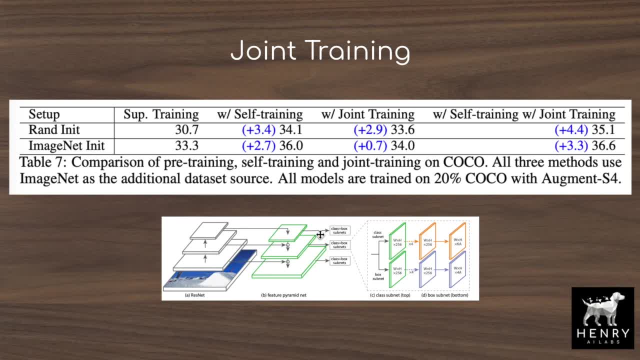 We can also get gradients through the limited COCO data set and we can still use this to do the pseudo labeling of the additional unlabeled data and use all these different multitask tasks to perform the loss and update the network. The author's reason that the success of self-training is because it aligns. 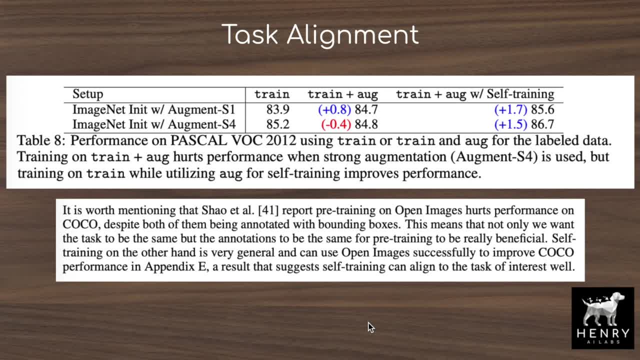 the unlabeled data with the labeled data in task alignment. So previous studies showed that pre-training on the open images, labeled labeled images with bounding boxes, doesn't necessarily improve performance on COCO. even though they are the same task with the same kind of labeling, there still is this distribution. 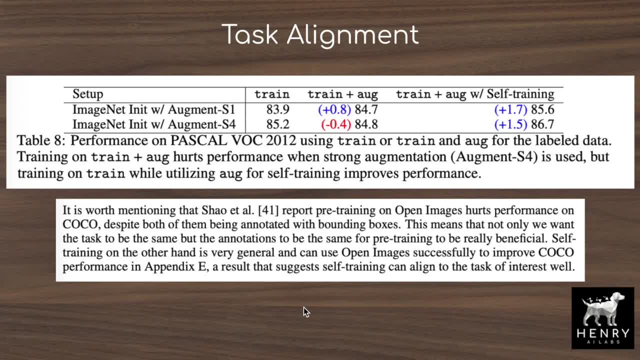 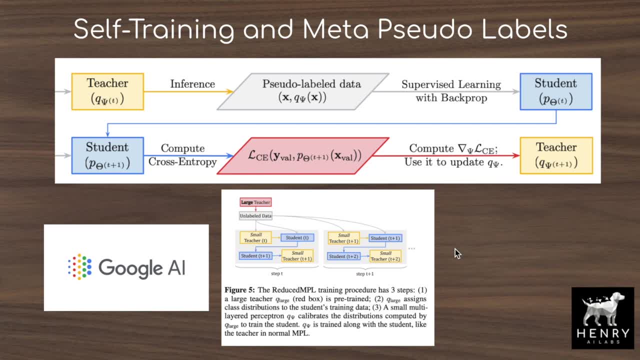 correction with respect to the annotation that pseudo labeling helps to correct. Meta-pseudo label serves a similar purpose: to correct the label distribution that the student network is learning on, to align the task of the unlabeled data and the labeled data and to facilitate learning. 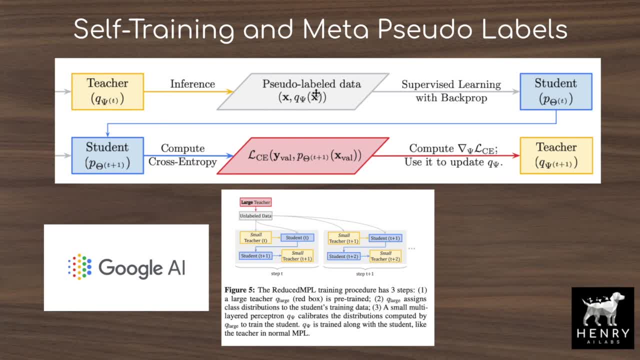 This is another interesting way of formulating this paradigm of having this pseudo label distribution in the case of self-training or using the previous model to label the data, and in the case of meta-pseudo labels, we're going to use this gradient, through a gradient meta-controller operation, to control the label distribution as well. 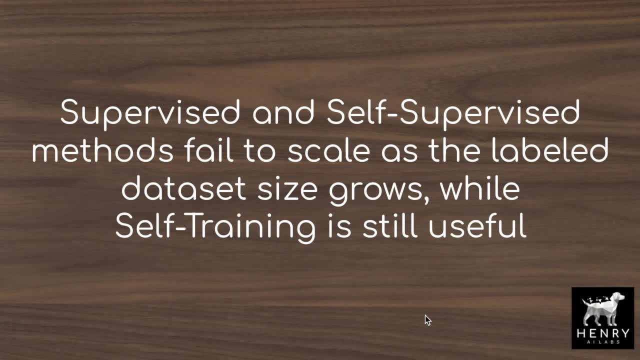 Some of the key takeaways from the study are that supervised and self-supervised learning fail to scale as the labeled dataset size grow, as we saw by going from 20 percent to 40 percent, up to 100 percent of the dataset, And it doesn't increase the performance. 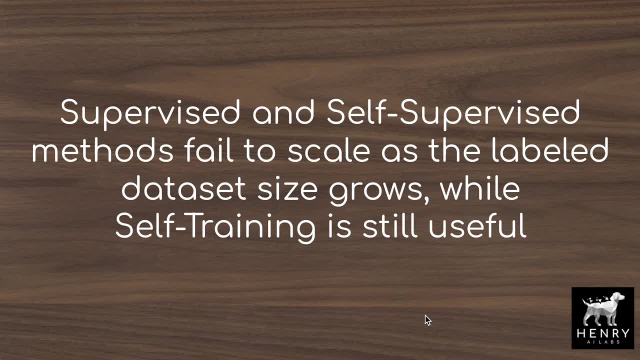 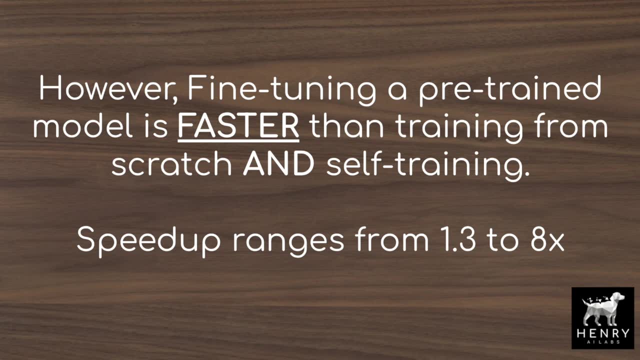 while you're increasing the level of data augmentation. But self-training is still useful in these settings. But fine tuning a pre-trained model is still faster than training from scratch and self-training. Self-training is this iterative algorithm to train a model from scratch, using it to label this unlabeled dataset and then 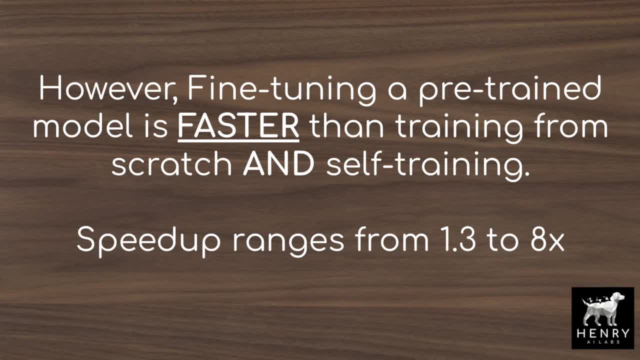 training a new model on the combination of those two datasets. So that's more time consuming than, say, fine tuning a pre-trained model that's been trained with supervised learning or self-supervised learning And they know that the speed up can range from one point, three to eight times faster. 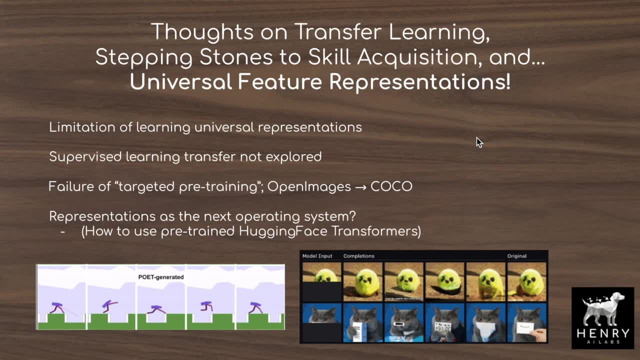 The results from exploring pre-training and self-training show that we still don't have these universal feature representations or features that we can get by pre-training on ImageNet, supervised learning and then taking those features and using them for classification on a different image dataset, bounding box detection or, say, semantic segmentation. 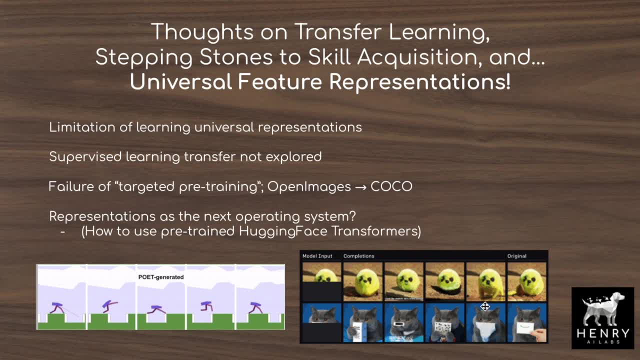 OpenAI recently explored the universal feature representation capabilities of a generative model with 6.8 billion parameters. They train this model to autoregressively predict the next pixel, and do this at scale, and then try to take those representations and use them for ImageNet or CIFAR 100 classification. 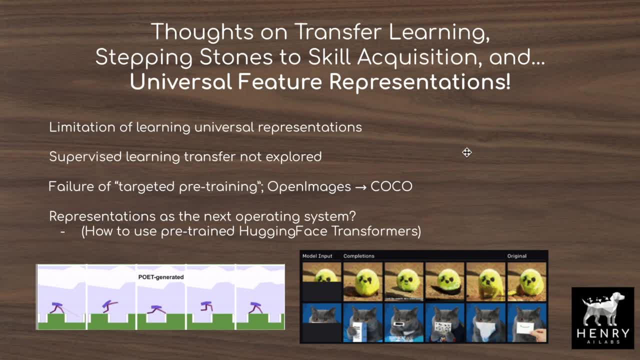 But even in this case they don't surpass, say, the state of the art with supervised learning and things like self-training with Noisy Student on those datasets. So we still don't have this universal feature representation that we can get by leveraging extra data and then have this one almost operating. 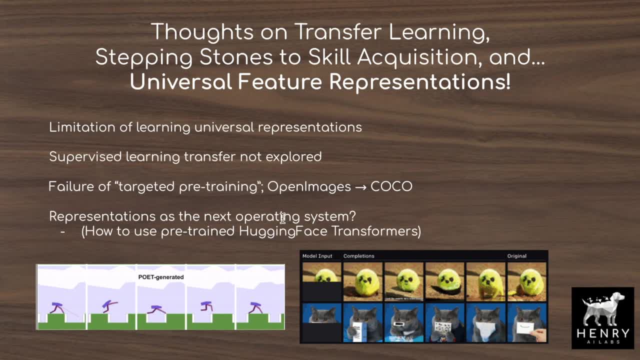 system representation, where we just take this representation and use it as features for all of our different downstream tasks. So it's kind of interesting to think about how we're going to fine tune representations, leverage, pre-training and extra data. So one of my favorite papers is Poet. 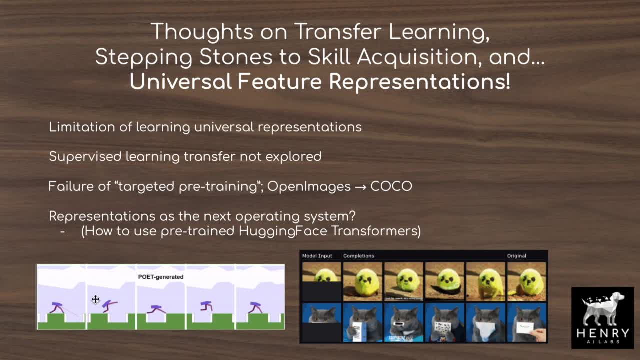 Poet is exploring this stepping stone curriculum, as this bipedal walking agent controller learns how to control the walking agent across a really complex terrain with maybe all sorts of different bumps and ditches, And so this curriculum evolves to create this complex controlling walking behavior. 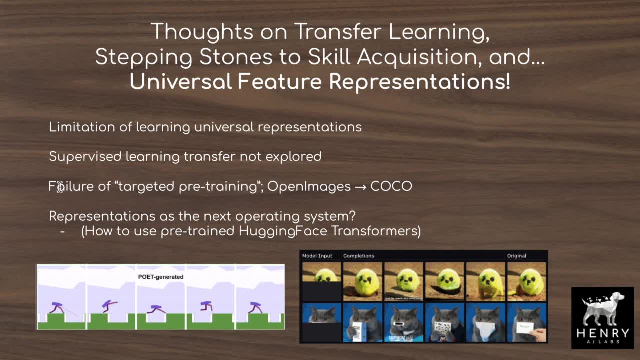 So I think it's interesting to think of these pipelines as we go from pre-training on, maybe, supervised learning, pre-training with self-supervised, contrastive learning, generative modeling, all these different ways that we can think of chaining different tasks to learn these representations. 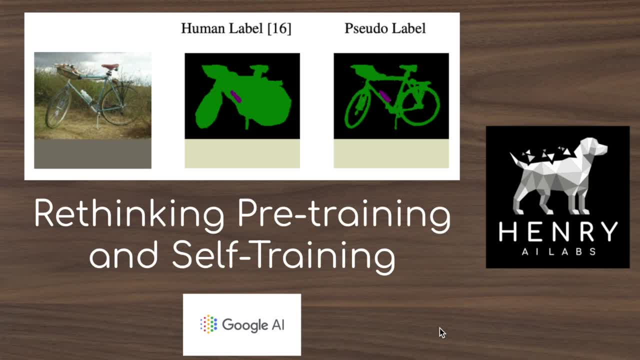 Thanks for watching this overview of rethinking pre-training and self-training. Hopefully, from this video, you'll get a sense of what self-training is and how it's different from supervised or self-supervised pre-training, and how it's being adapted to do bounding box. 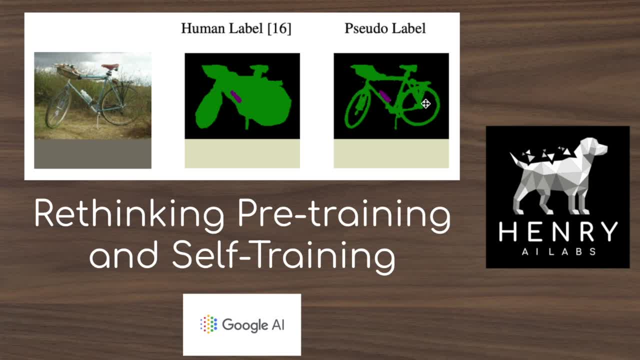 detection or semantic segmentation. This study shows that self-training is outperforming pre-training with respect to adding more data augmentation and more labeled data for the downstream fine tuning task, in the case of comparing it with supervised learning on ImageNet and self-supervised learning. 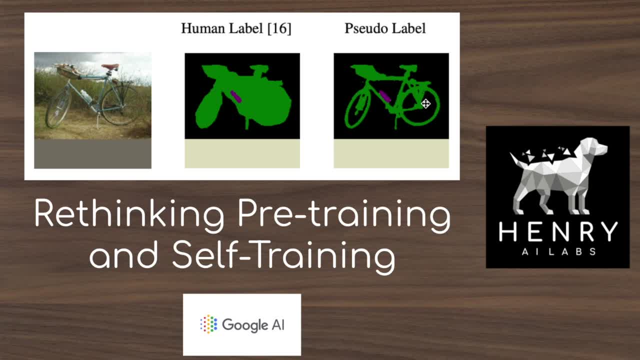 with the SimCLR framework. Thanks for watching And please subscribe to Henry AI Labs for more deep learning and AI videos. Thank you for watching.